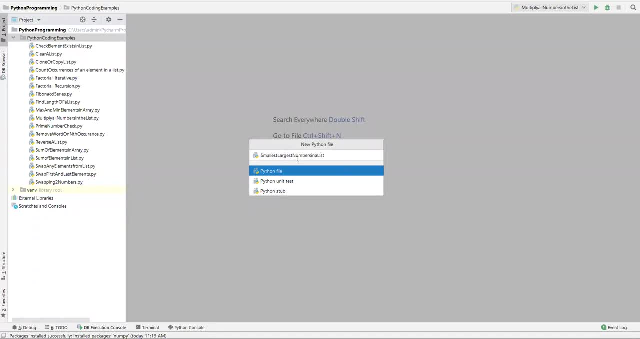 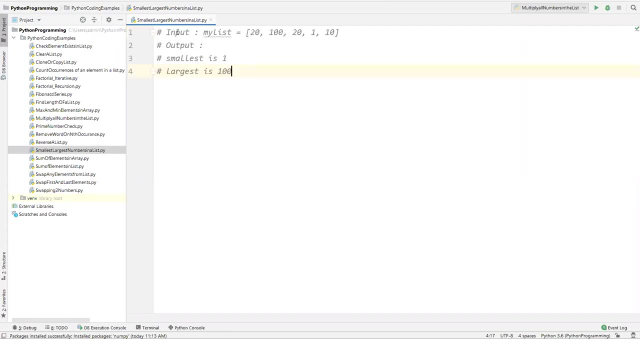 I will name it as smallest. largest numbers in a list. Let's take a Python file. So here let's see multiple approaches, So I'll show you the first approach. I have a my list here which contains some of the values, and smallest is one, largest is 100. I need to find out. So the first approach is: 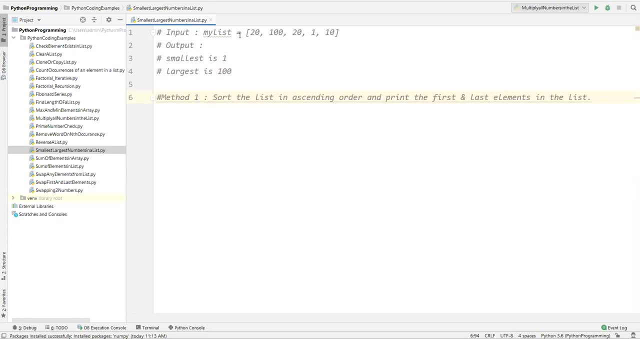 in the first approach we have to sort the list here. So we have to sort in ascending order, we have to sort the entire list in ascending order And to do this we have a directly method is available: sort method. So by using the sort method we can directly sort the elements in a list. After sorting the list, 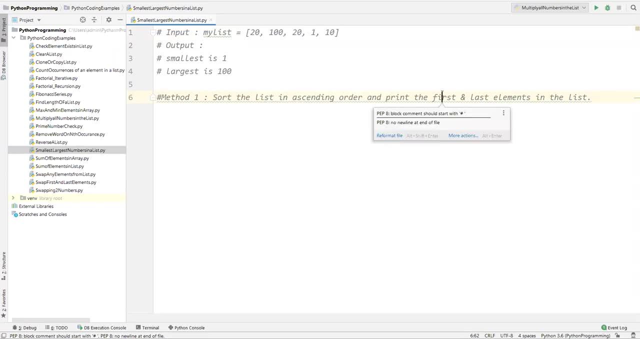 then we can extract the first element, which is obviously the lowest element, then extract the last element, that is obviously the greatest element, or largest element, right? So let's see how it works. can do this. so here I will define my list equal to, and here I will add some. 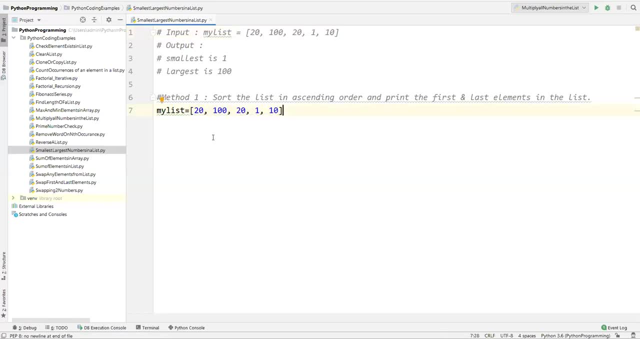 of the values. let us have these values. so 20 hundred, again 21 and 10. so these are the current values I have. so first of all let us sort this particular list. so to sort this particular list we have to say my list, dot, sort method and this: 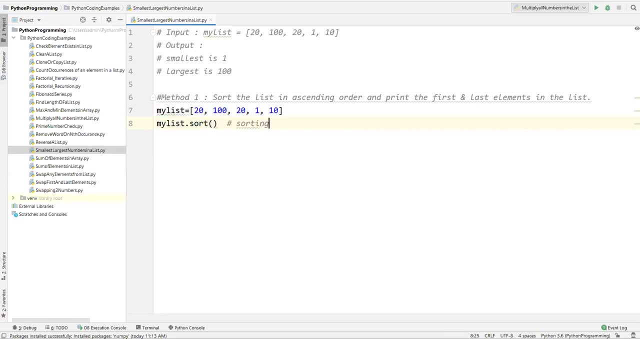 method will sort the elements. so here this is basically perform the sorting. so after sorting I'll just print my list as it is now, just observe how it will be sort. so when I run this code so it will print sorted numbers, okay, so this will print exactly the same way. so this is a sorted element. so from these sorted 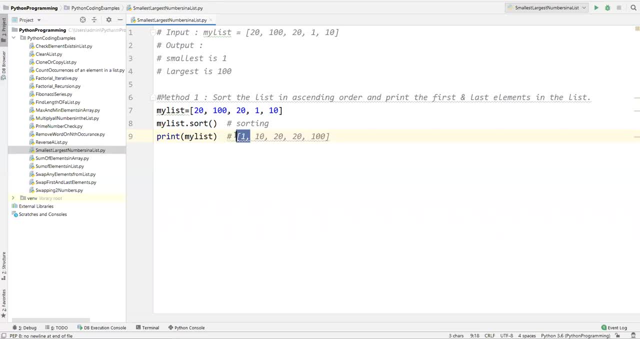 elements. just, we need to extract our first element, which is the lowest element or smallest element. then we have to extract the last element, which is a largest element. right now how we can extract the first element and the last element. so to start the first element, we can simply say: let me just print here the smallest. 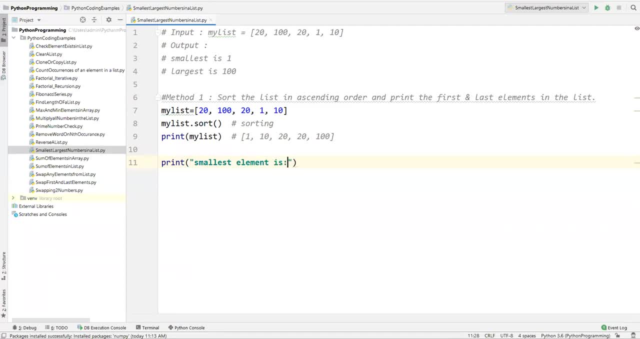 element is, the smallest element is- and here from my list, my list- and says say 0, 0 is a starting index, so starting element how we can access by adding the 0 index. so every element is having index. so index is always start from 0. so I'm 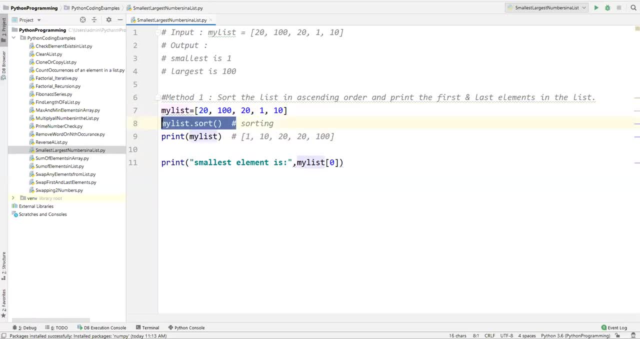 extracting 0, so 0 means he currently 1 is there after sorting. these are the element. so the first element is 1, so this will print 1 here. this is a smallest element. now, similarly, if I want to extract the last element in this list, 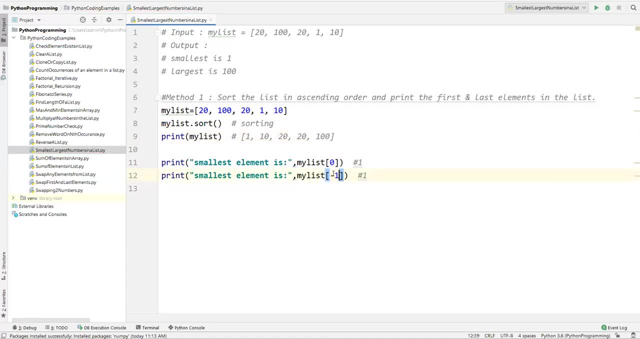 so we have to say minus 1, so minus 1 is representing the last element. so last element from this sorted list. now, this is a largest element, the last element will be the largest element and and it should be 100. now when I run this code it will print: so these are the. 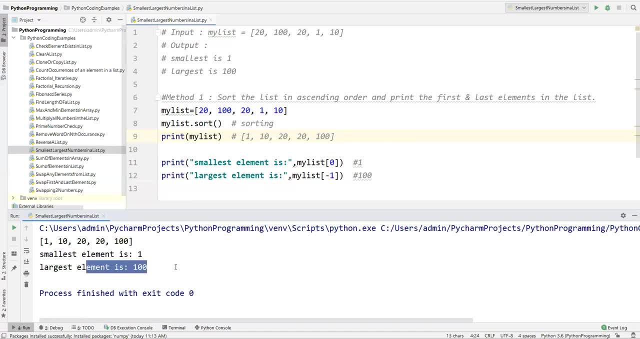 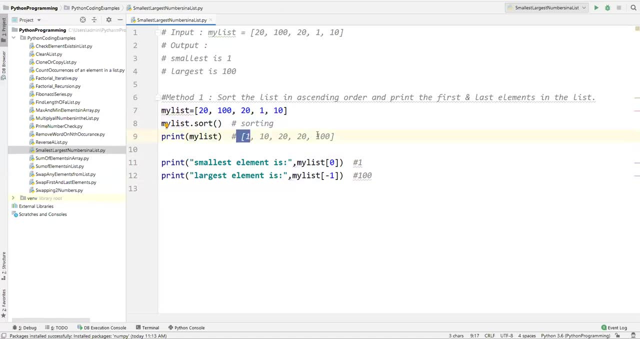 sorted list and smallest element is 1 and the largest element is 100. now, this is a one approach. we can first sort this list and then we can extract the first element and the last element. they are obviously the smallest element and the largest element. so, apart from this, we also have built-in methods and mean and 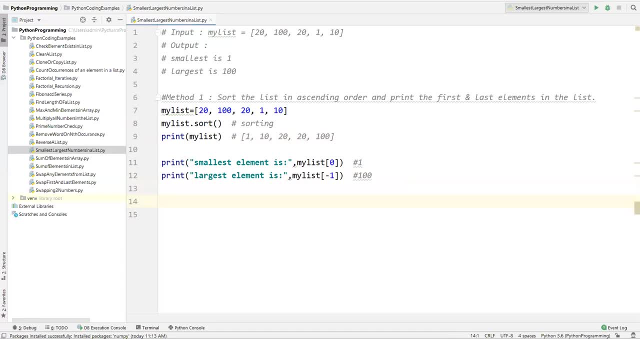 maximum methods. they are straightforward. now I'll show you one more approach by using mean and maximum methods. so I'll just comment this now again: define the list which contains some of the elements. now here we don't need to sort anything, ok, so simply we can say: print and here: 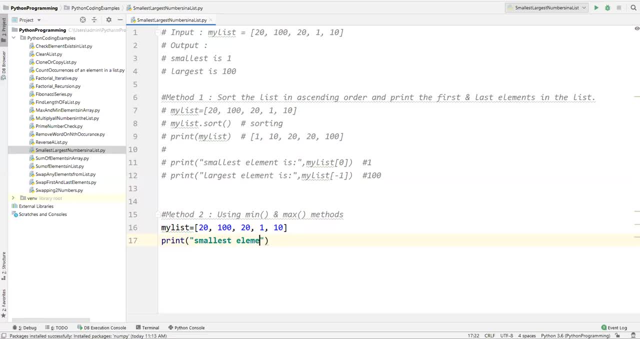 I'll say smallest element. smallest element is: you can simply say mean off min. so mean off. specify the list variable. I'll say minus 라는 flaco. ok, let's say your smaller them in my list. so that's it. from this, my list. this method will find out which one is. 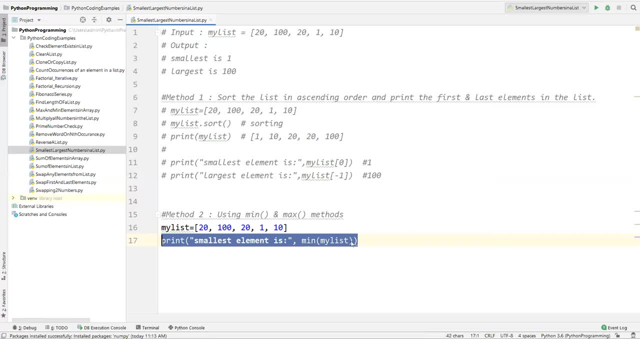 the lowest or smallest element and it will print here. and similarly, if you want to extract the maximum element, you can also get it. but they can say largest element, max or largest element. we can use max method here, M, a, X, max of my list. so mean is a method which will find minimum element which is smallest. 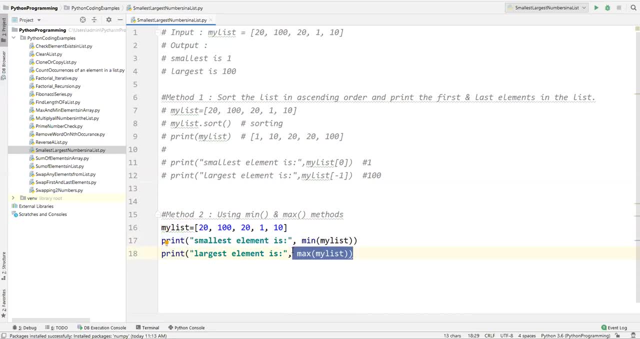 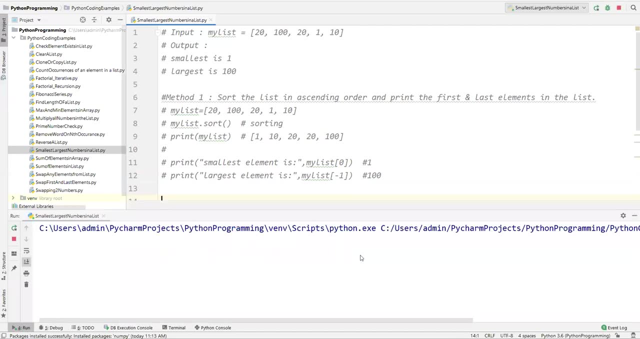 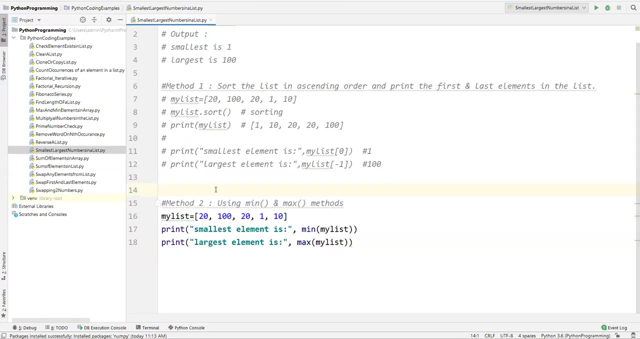 element from this list, and max is another method which will find a maximum element which is the largest element in the list. that's it now. let us execute. now it prints: the smallest element is one, then largest element is hundred. okay, so this is another approach. okay, so we can find the.